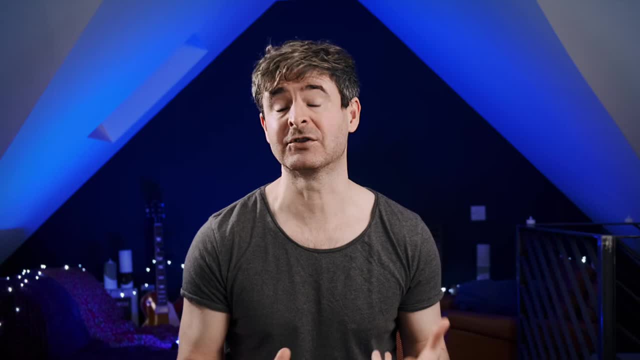 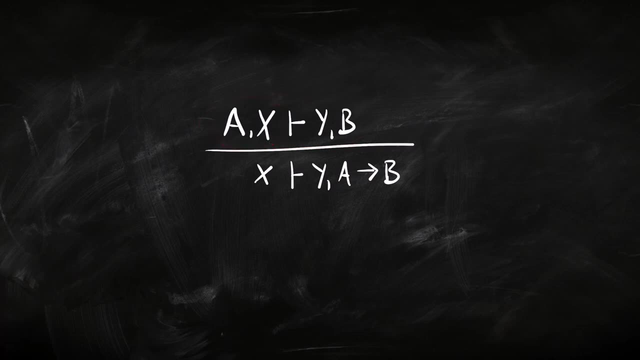 in the first place, let's just look at some sequent calculus rules. Here's a typical one, Okay, so what's going on here? So, looking above the line, we've got some sentences on the left, and then we've got this kind of inference sign and we've got some sentences on the right. Okay, so maybe we're thinking that 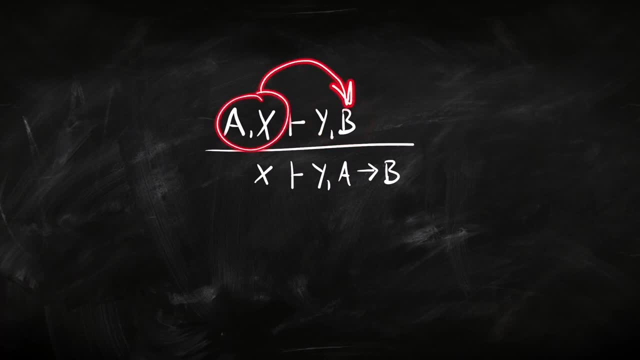 we're talking about these sentences, proving these sentences Okay, but we've also got some stuff above the line and some stuff below, And in a proof rule we normally think of that as meaning: well, given some stuff above the line, we infer the stuff below the line. 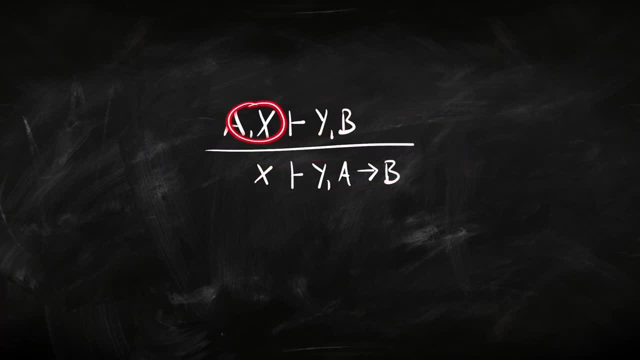 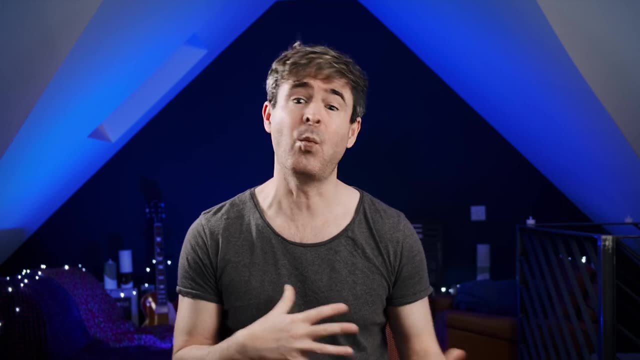 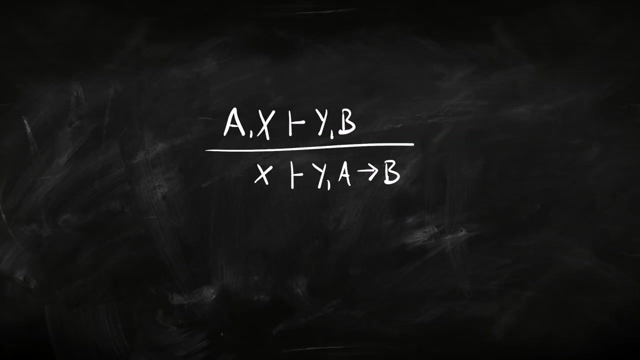 Okay. so are we talking about inferring from this lot to this lot, or are we inferring something up here to something down here? Which are the premises and which are the conclusions? That's the first difficult thing to understand with these sequent calculus rules, And the second difficult thing to 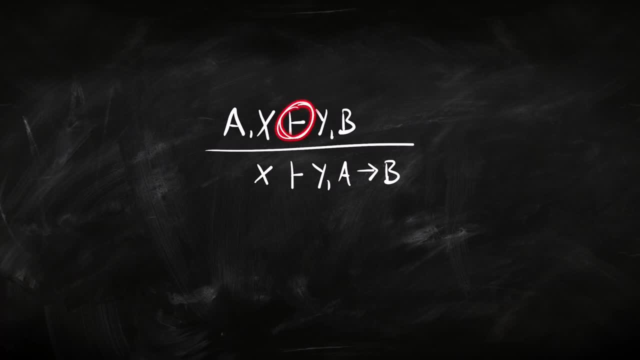 understand about a rule like this is: here's our inference sign. So we were going to get some things that are really simple. So we would expect to have the premises on the left and the conclusion on the right, But on the right we've also got a bunch of sentences. We've got multiple conclusions. What exactly does? 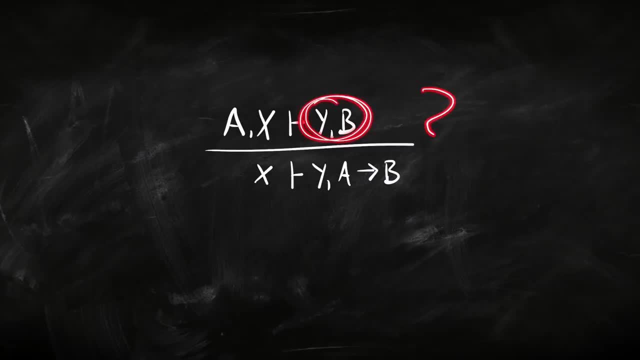 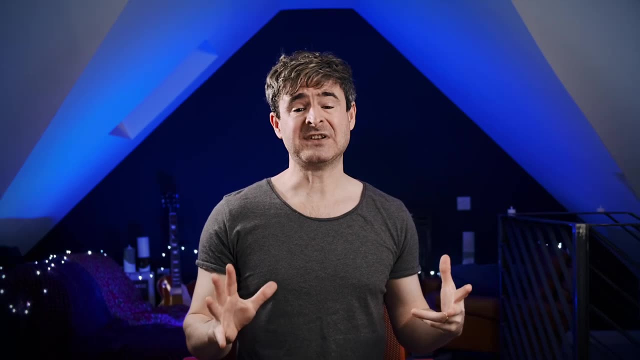 that mean: How do you infer multiple things from some premises? So I'm going to tell you how I got my head around understanding rules that look like this. To build up to this, what I'm going to do is I'm going to start off with some really, really simple proof rules and we're going to think a 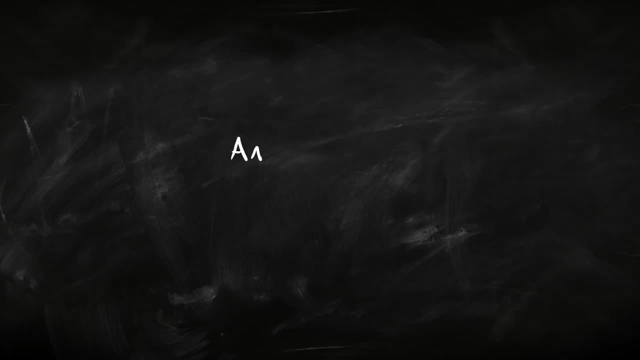 little bit more about what are we really doing with them. So let's take one of the simple rules. So let's start off with the simplest rules of all: Conjunction elimination. So we start with an and a and b, and if we've got that in our proof, we can infer a on its own and we can infer b on its own. 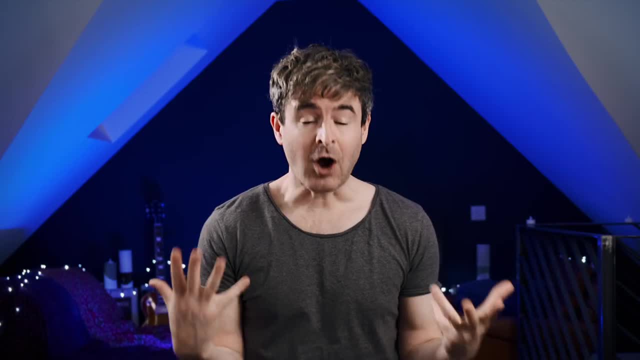 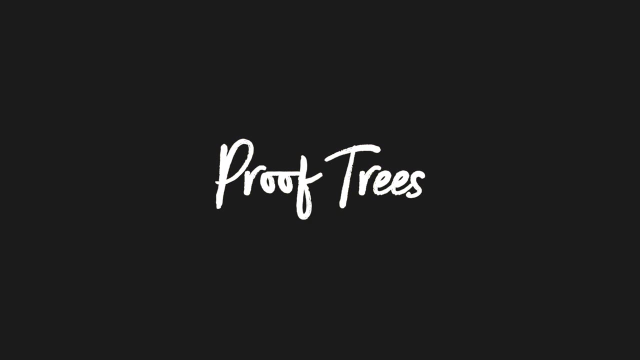 Okay, couldn't get simpler than that. Now, exactly what we're trying to do in inferring sentences like that depends on what kind of proof system we're doing. So think for a moment about proof trees. If you don't really know how proof trees work, go and take a look at this video up here. 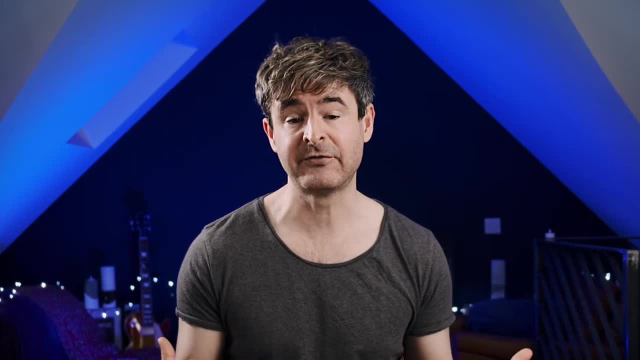 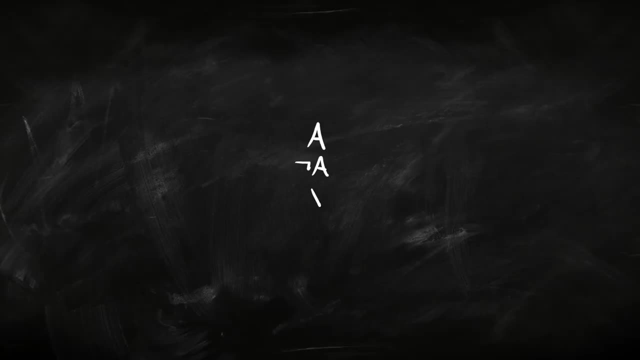 I'll give you a quick explanation there. What we're really trying to do in a proof tree is close our branches- and typically we're closing a branch when we see a sentence and its negation. Effectively, we're saying: we've got a, we've got not a. that's bad, something's gone wrong- close. 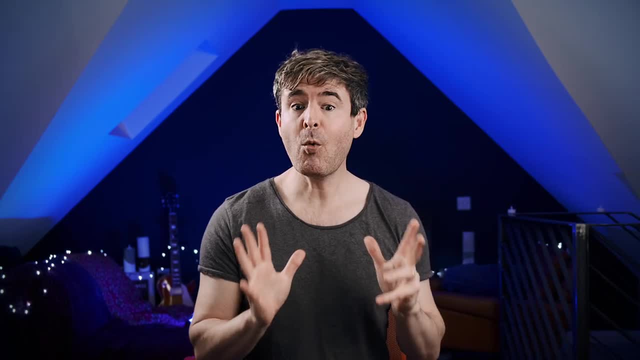 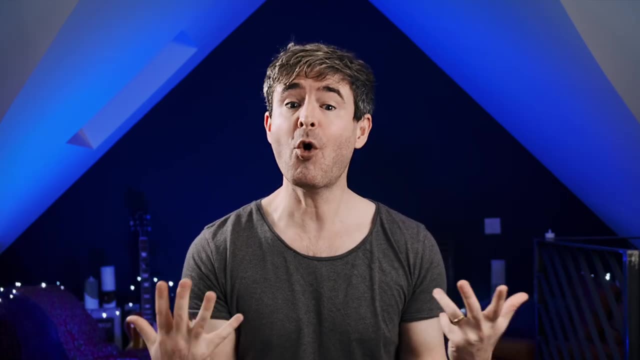 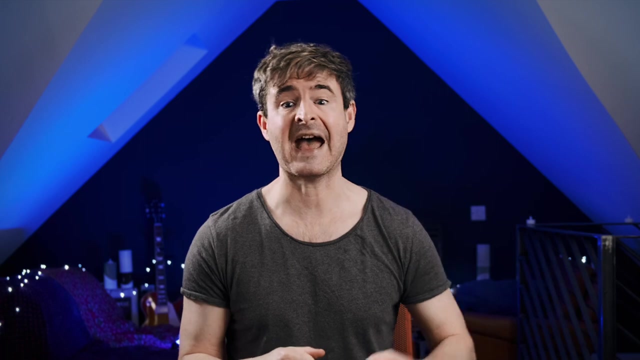 that branch and if we close all the branches, we've got a proof Now that all works fine and good in logical systems where there's a problem with having a sentence and its negation. But not all logical systems are like that right, If we're working with a paraconsistent logic, maybe it's okay to have a. 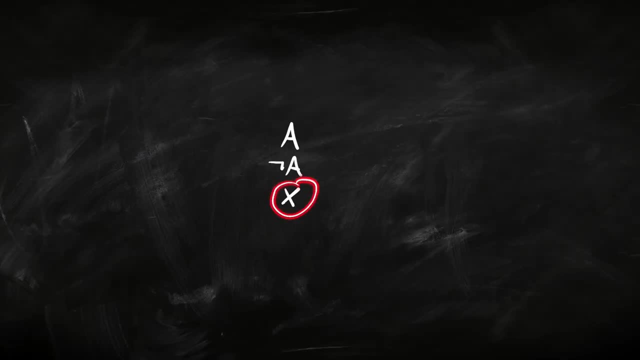 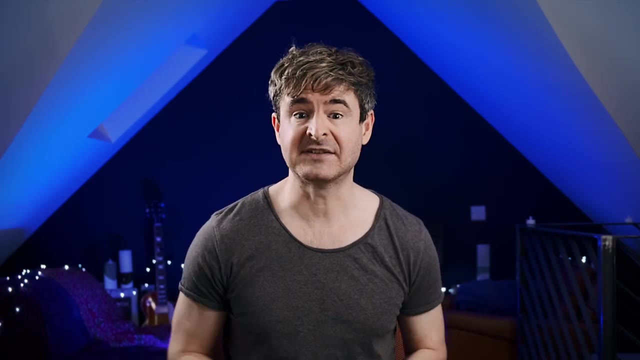 and not a on its own Also. so we don't want to assume in our proof system that that's going to be a bad thing. We want that to be an optional rule. So instead of taking a and not a to be as bad as it gets, 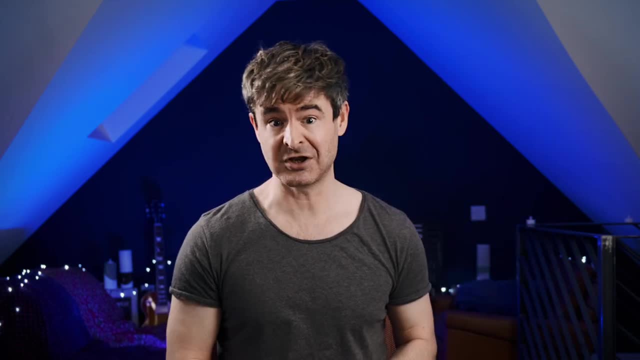 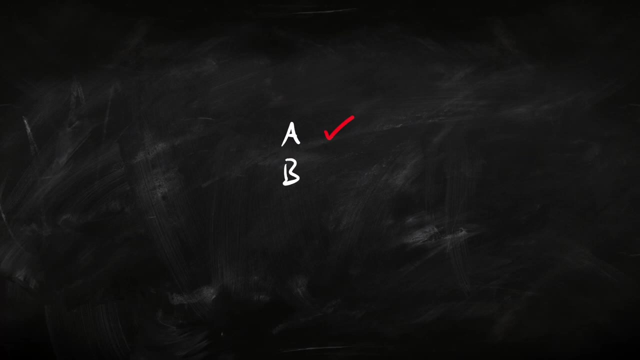 what we could do is we could have a way of marking the sentences that are good and the sentences that are in some way bad. So, for instance, we could tick the sentences that we like or those that we accept and we could put a cross by the sentences that we don't like or those that we reject. Okay, 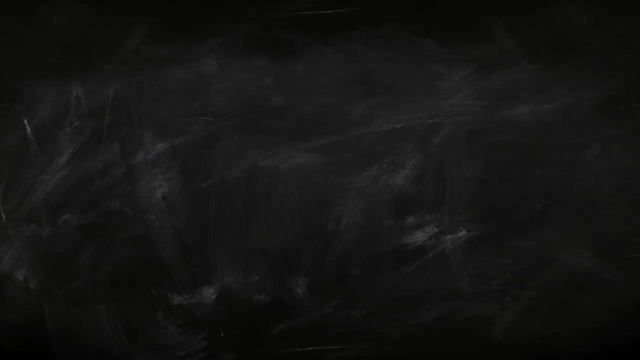 so in the case of our really simple rule of conjunction elimination, what we could say is: if we tick a and b, if we put a tick by a and b, then we can extend the proof with an, a and a tick, and we can also extend the proof with a, b and a tick, and then we would say, kind of in parallel with the: 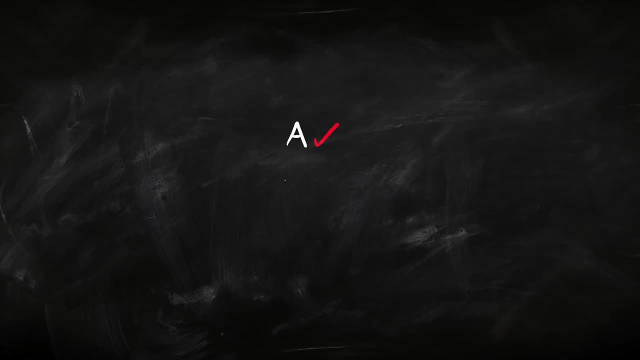 proof tree case. we've got a problem when we take some sentence and we put a tick and a cross by it. Something's gone wrong there, and that would be like closing the branch and saying, yeah, maybe we've got a proof there. So this works great with simple rules like conjunction. 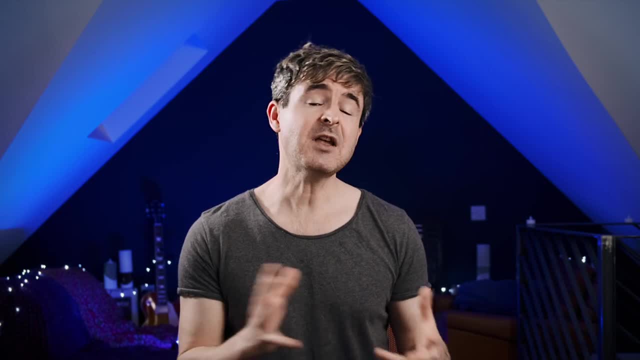 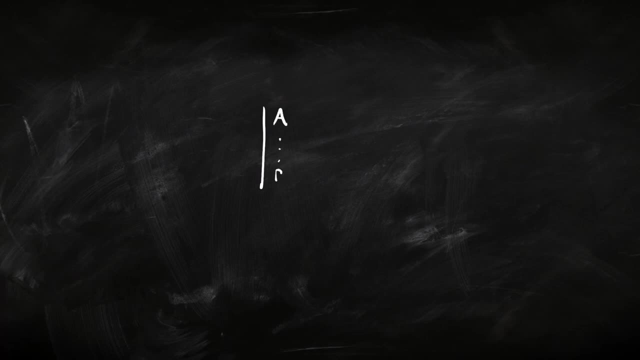 elimination. but not all rules are going to be like that. So think about how you infer an implication: if a then b. Typically, what you're going to do is you're going to assume a, try to reason to b, and if you can do that, then you've inferred: if a then b. So in other words, we're working there with a bunch. 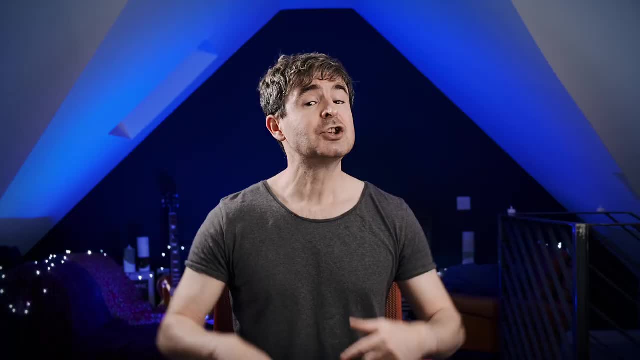 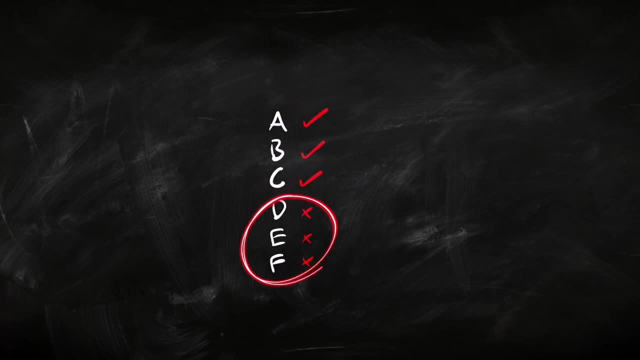 of sentences, not just individual sentences. So what we might want to do is have some way of tracking. these are the sentences that I like, that I've ticked, that I accept, and these are the sentences that I don't like I've put a cross by. I reject those. We can write down sentences, the ones we 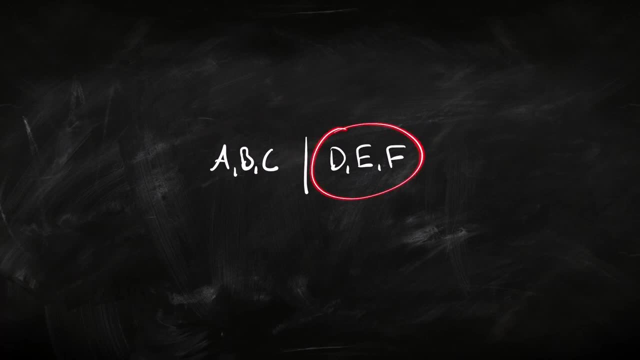 like, or the ones we accept on the left and the ones that we don't like on the left and the ones that we don't like, the ones we reject on the right. and we can say, given we've got a proof like this, we can extend it with stuff on the left that we like, like this and stuff that we don't like that we reject. 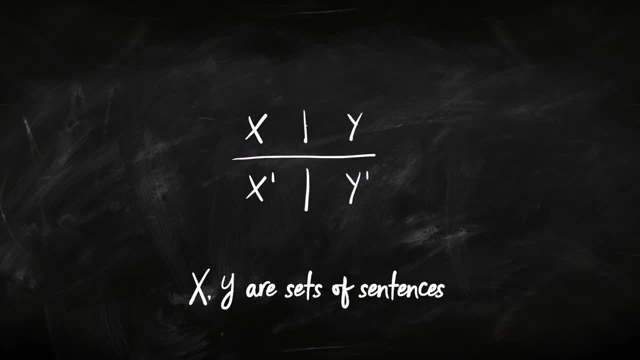 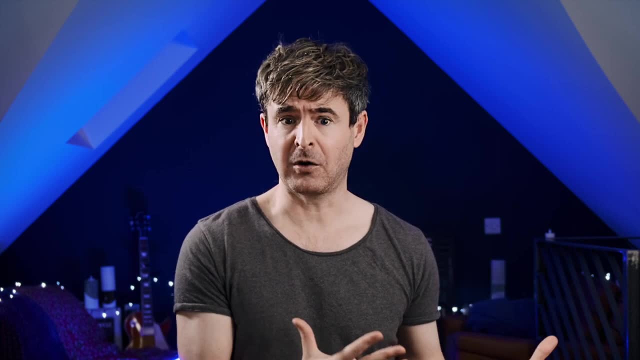 on the right like this, And now we're getting closer to what our sequent calculus rules look like. So if we're going to think about rules in this way, what would a proof look like? What is our aim in a proof? Well, think back to the proof tree system, right? we're trying to show that something's. 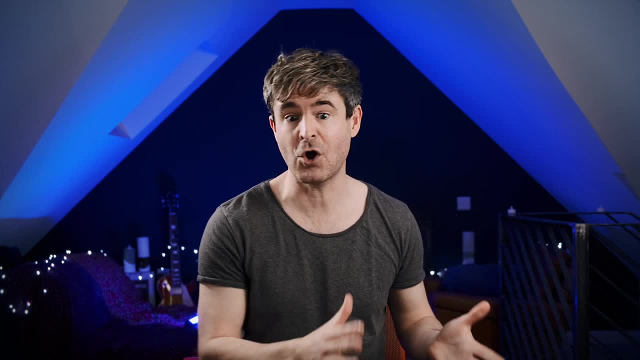 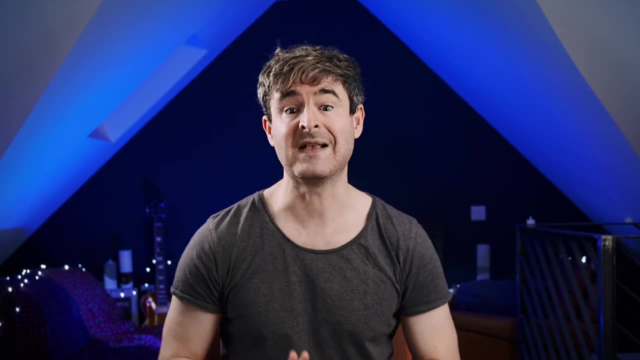 gone wrong. a bad thing has happened, like p and its negation, not p In our new system. what we really want to say is: there's something bad about liking this stuff and also not liking this stuff, or there's something bad with accepting this and rejecting this stuff over here, And the thing that 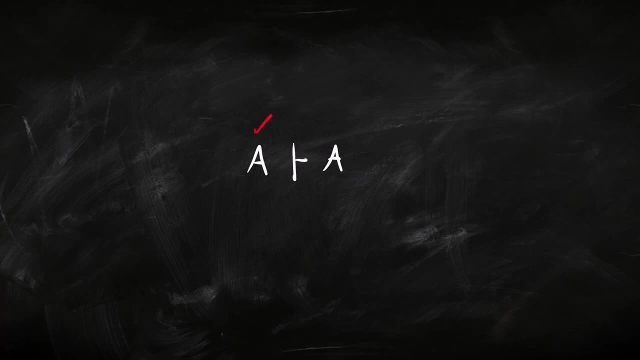 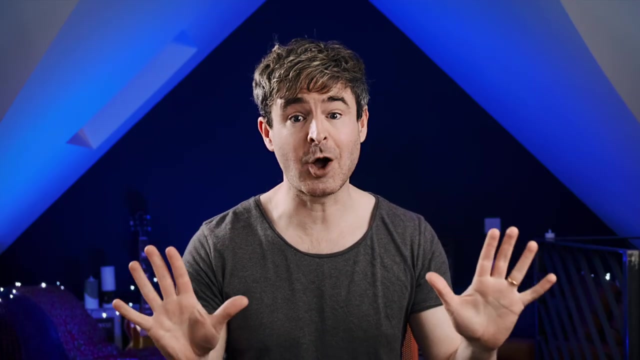 you mustn't do. rationally speaking, logic is: accept and reject the very same sentence. a- So this kind of thing is as bad as it gets. we're going to start proofs with that and whatever we can infer from that, we're going to reject. So we're going to start proofs with that and whatever we can infer from that, we're going to reject. 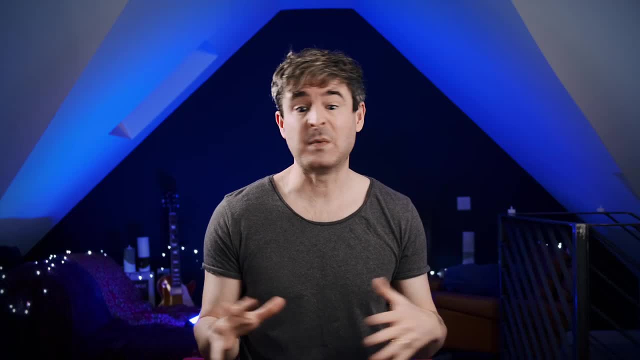 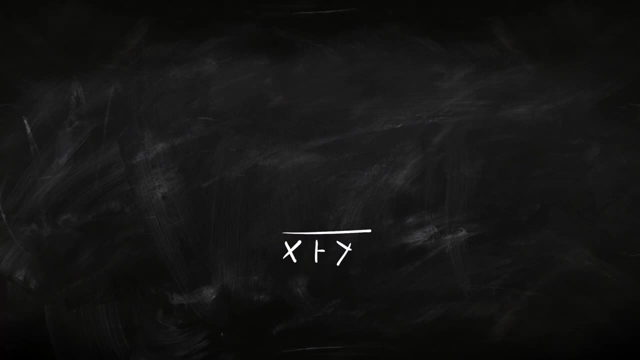 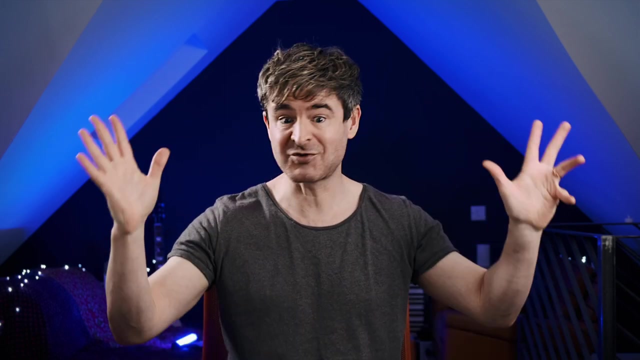 going to count as approved sequent. Now, in practice we don't do sequent proofs from top down. what we do is we start off with what we want to prove at the bottom of our sheet of paper and we work upwards. We might build a tree, the way trees actually grow, from the root up to the 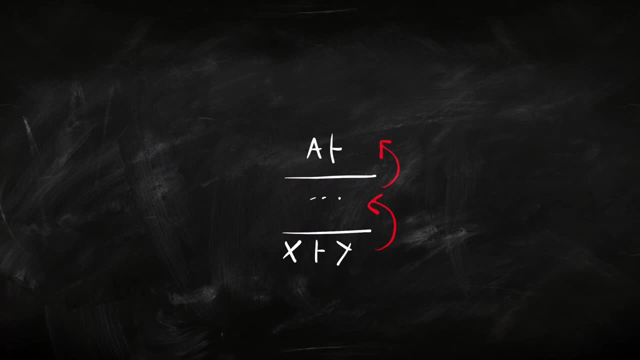 branches, and what we're going to want is one of these really bad things: accepting and rejecting the same sentence at the tips of all our branches. If we've done that, then we've proved the thing that we start off with. so, with this understanding of a sequent sentences on the left that we accept, 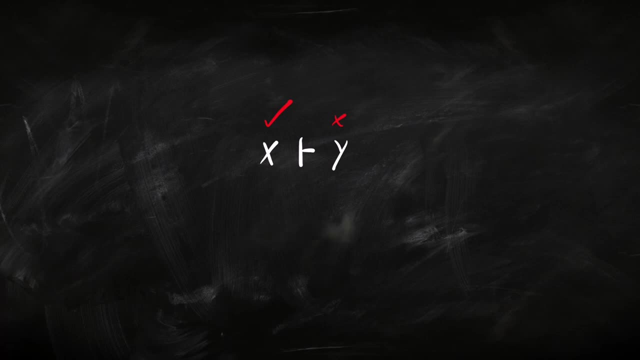 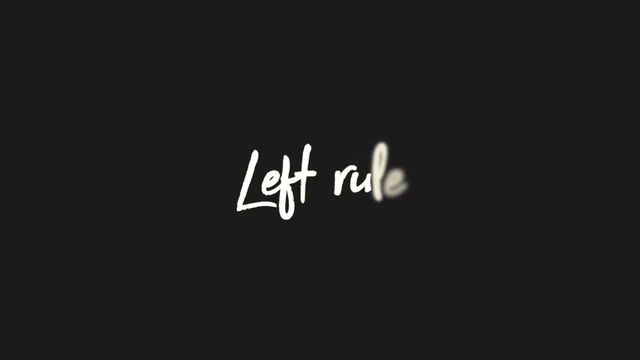 and sentences on the right that we reject. how are we going to formulate a system of rules? All our rules are going to be introduction rules showing how to introduce that connective, and we're going to have one rule for that connective over on the left as something we accept and we're going to 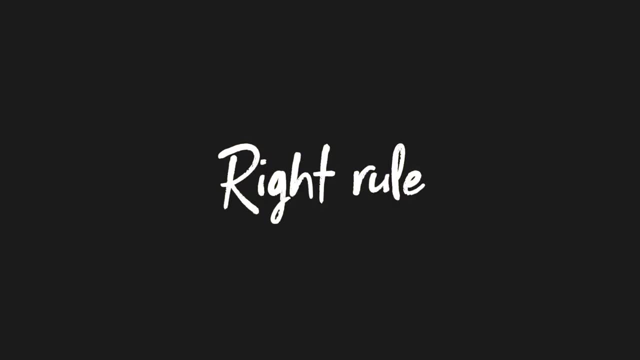 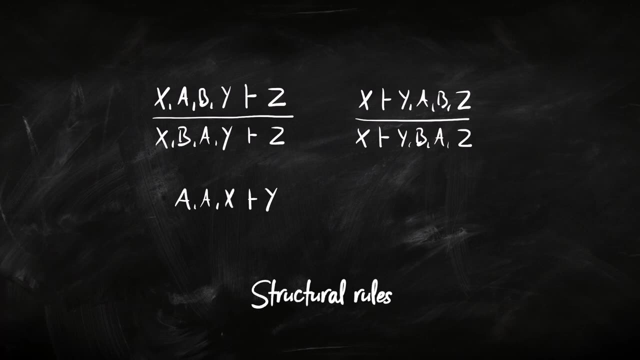 have one rule for that sentence over on the right as something we reject. There's also a bunch of structural rules that say things like: it doesn't matter which order you write the sentences down in, it doesn't matter if you repeat sentences, We just have to make sure that the sentence slip into the right one. 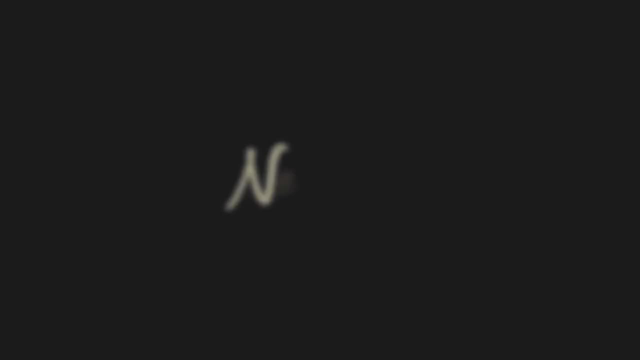 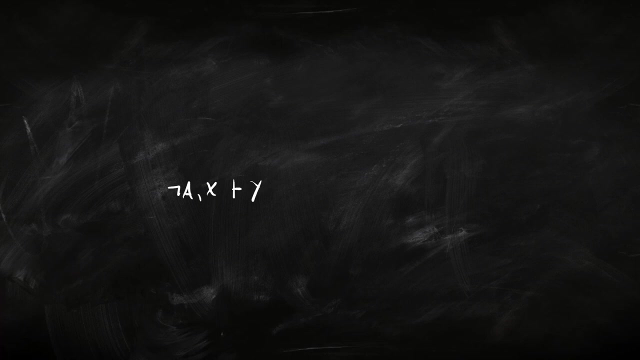 going to ignore those for now and just think about some logical rules. So let's take the case of negation. What should the rules be if you accept a negation? Well, if you like not A, then you shouldn't like A. So if you accept not A, you should reject A. So in other words, 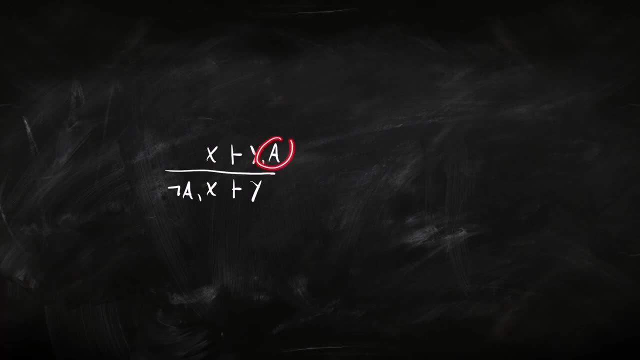 we should be able to move not A from the left over onto the right where it becomes A, And vice versa. right, If you reject not A, then you should be able to move that over to the left where it becomes A. So we can go from not A on the right to A over on the left. So here's another rule that 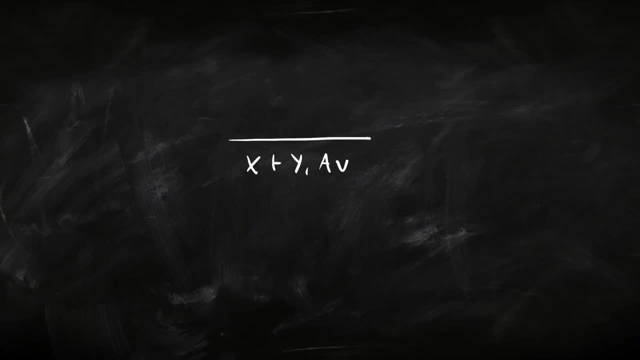 makes good sense within this framework. When should you reject a disjunction A or B? Well, you should reject it when you reject A and you reject B. If you can rule them both out, then you've ruled out A or B. So if you've got a whole bunch of sentences over on the right, 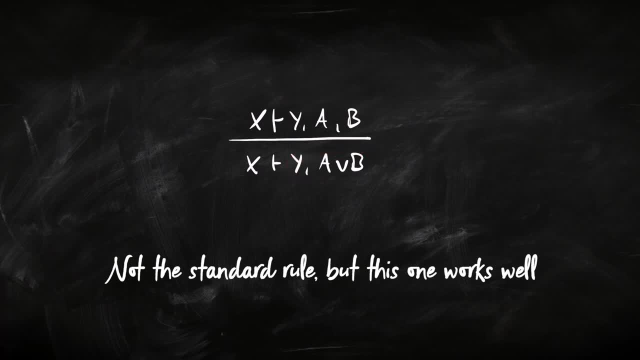 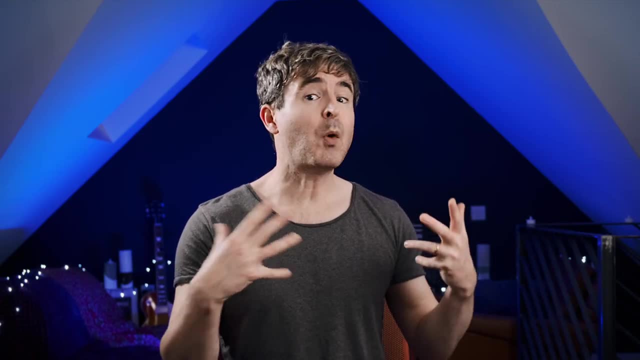 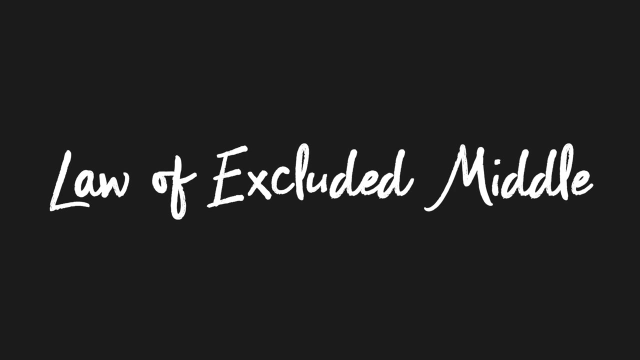 then you can put any two of them together with A or B, also on the right, as something you reject. Now, with only though those rules, we can already do some cool stuff. So I want to compare how we go about proving excluded middle A or not A in natural deduction, where it's really difficult, versus in the 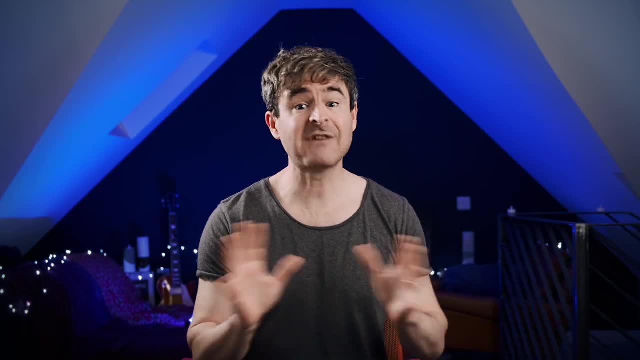 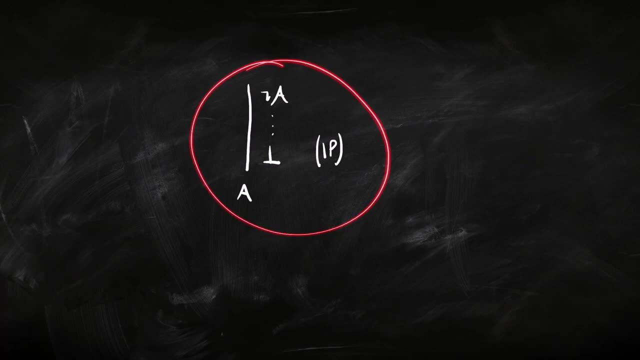 sequent calculus where it is super simple. Here's a really quick version of how it's going to go in natural deduction. To prove excluded middle in a natural deduction system we need to use proof by contradiction or indirect proof. So we're going to start off by assuming 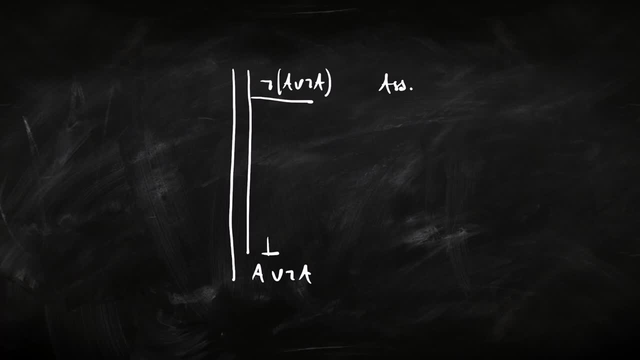 the negation of what we want to prove. So we start off with not A or not A. Then we're going to make a second assumption, A. From that we infer A or not A using disjunction introduction. That's a contradiction. so we infer the fulsome. We assumed A. 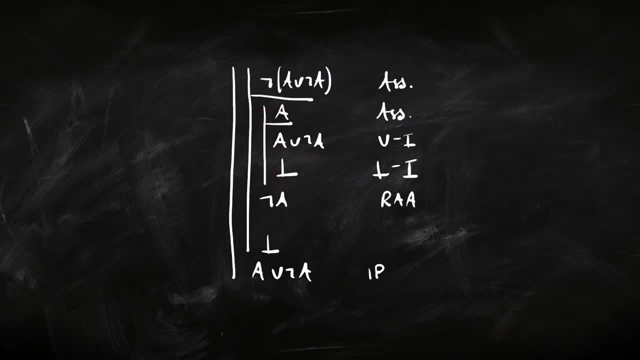 we infer the fulsome, so we can infer not A. From that and disjunction introduction we can infer A or not A. That's a contradiction too with our initial assumption that not A or not A. So again we infer fulsome. So from our original negated assumption we've derived a fulsome and using 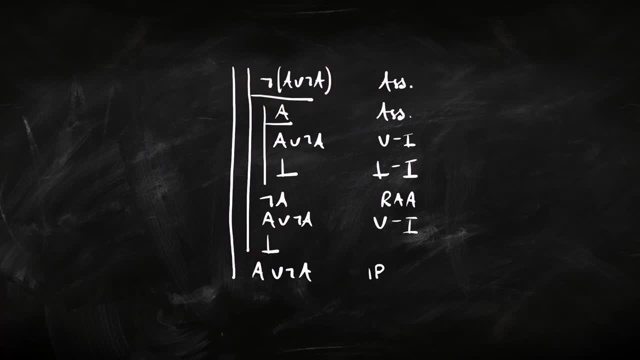 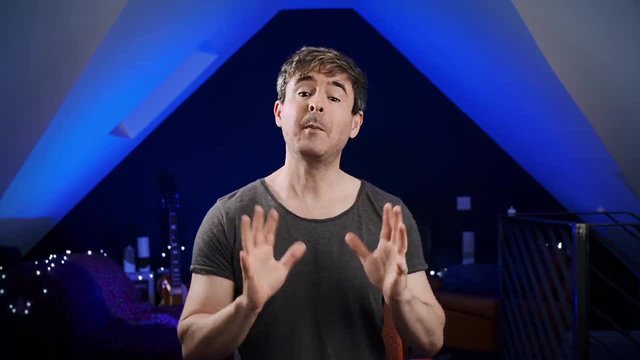 indirect proof we can infer A, A or not A. That's really, really complicated and it's not at all natural. So natural deduction doesn't do very well there, By contrast. here's how it's going to go in the sequent calculus: 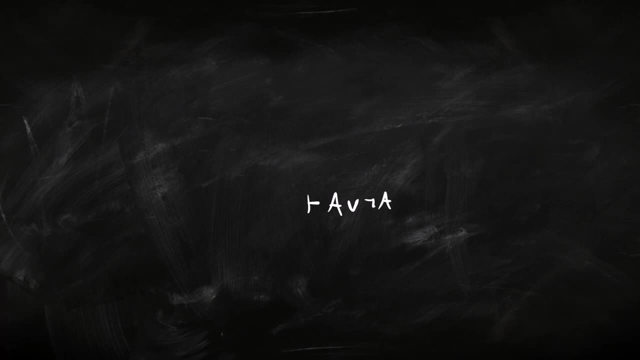 So we're trying to prove this: A or not A, which we interpret as rejecting A or not A. So if we're rejecting A or not A, then we're rejecting A and rejecting not A. Given that rule for negation, we can move not A over onto the left, and that gives us this: We've got a proof. 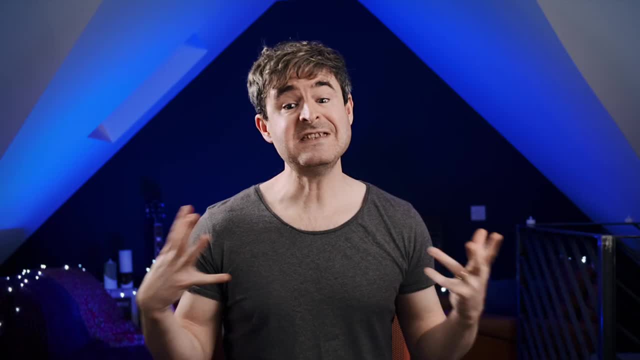 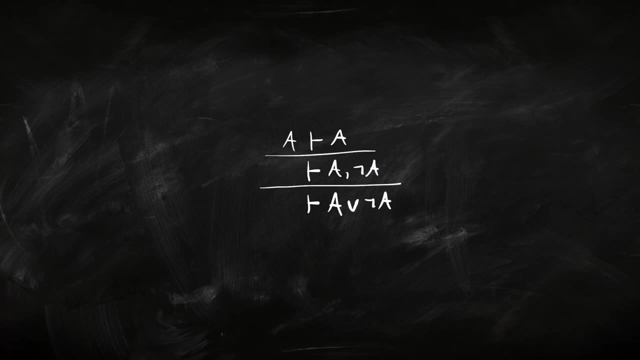 of excluded middle in three lines. I think it's a really nice feature of this proof system of the sequent calculus that we can prove this central feature of classical logic- A or not A- in such a simple and intuitive way. However, you might say, well, what about logics that don't have? 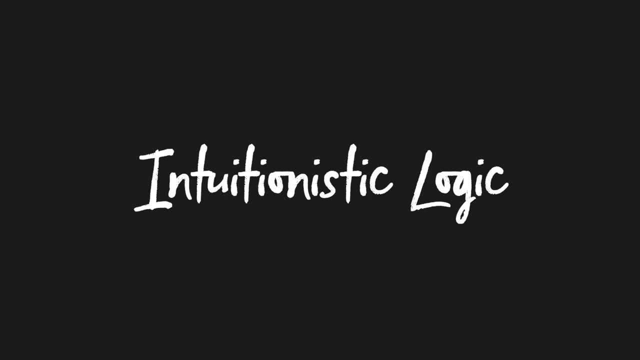 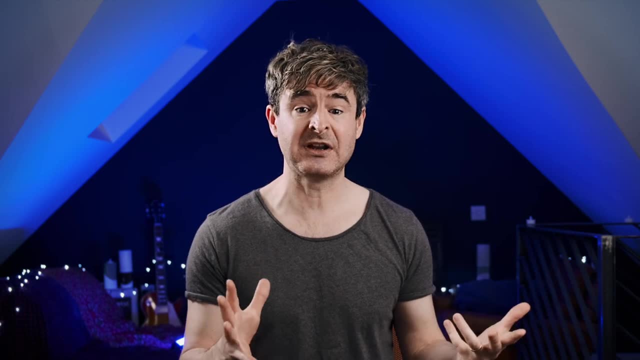 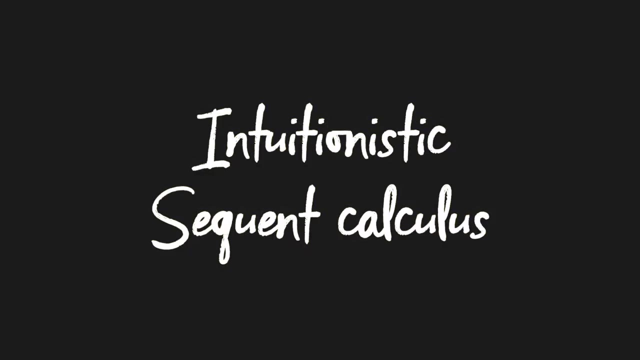 excluded middle, Things like intuitionistic logic. Is it going to be baked into this sequent calculus that we have to have excluded middle? So here's a second really cool feature of the sequent calculus: It's really easy to modify this system into an intuitionistic system which drops excluded middle. So again, let's just contrast this. 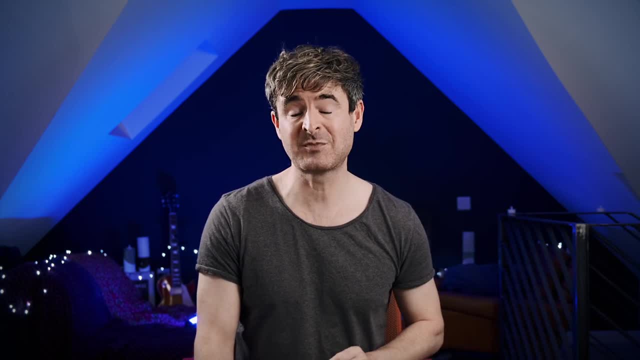 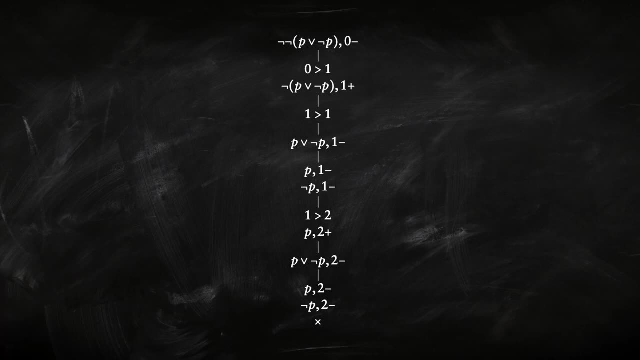 with a system like the tree proofs. If you want to do classical tree proofs, super simple, you can prove excluded, middle, no problem. But if you want to do intuitionistic tree proofs, they're really, really complicated. The rules are not intuitive at all, But in the sequent calculus it's really. 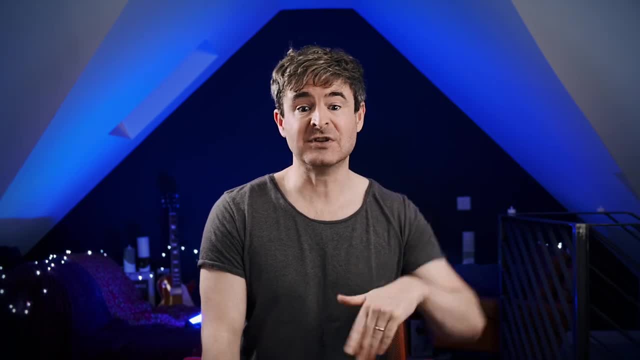 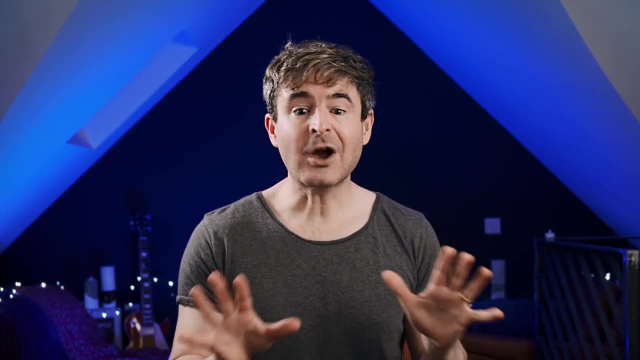 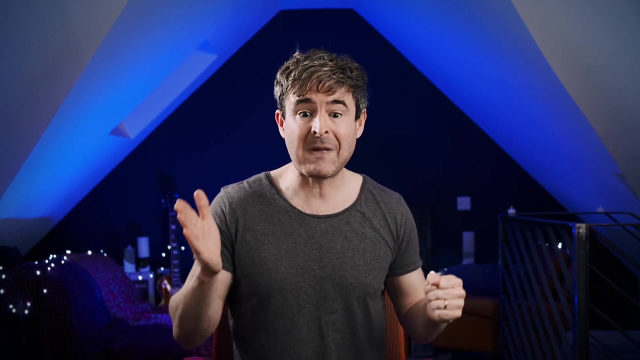 easy to go intuitionistic. All we need to do to block this proof that we did before is ban multiple sentences on the right. So we don't change any of the rules. We can still shuffle sentences from left to right, with negations coming and going. We've just got to make sure that. 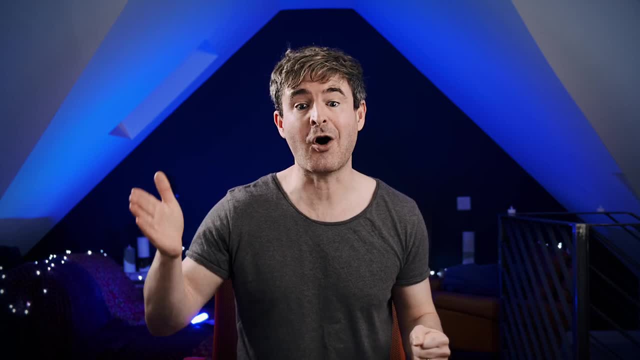 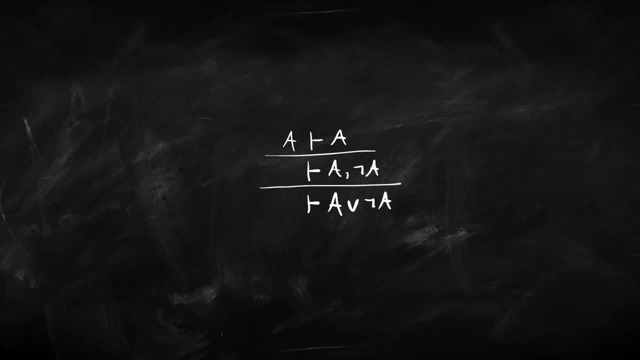 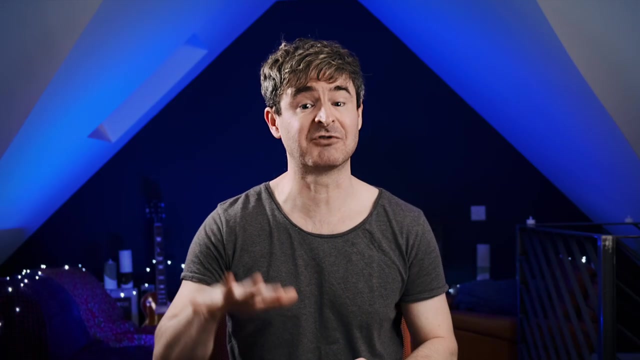 we never have more than one sentence over on the right And, if you think about it, that's going to block any attempt to prove excluded middle, Because the only way of getting A or not A is to have A, not A, over on the right. So we need two sentences on the right to prove. 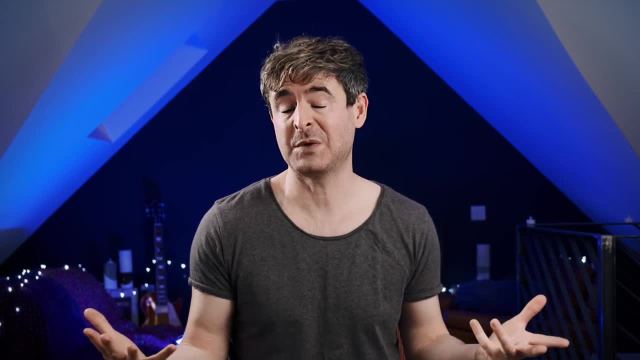 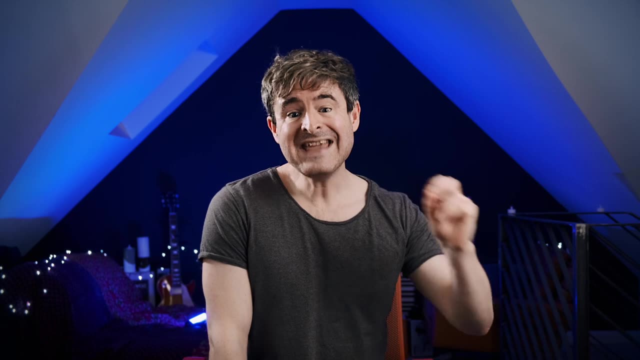 A or not A. We ban that and we've got an intuitionistic system. That's a really nice feature of this whole sequent calculus setup that we've got. So for me, the key to getting into sequent calculus is not to try to understand the rules in terms of this stuff, implying this: 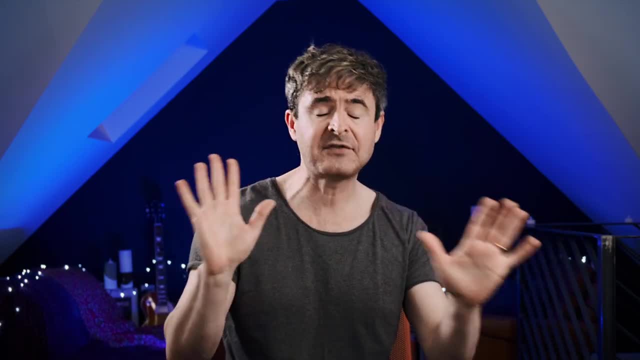 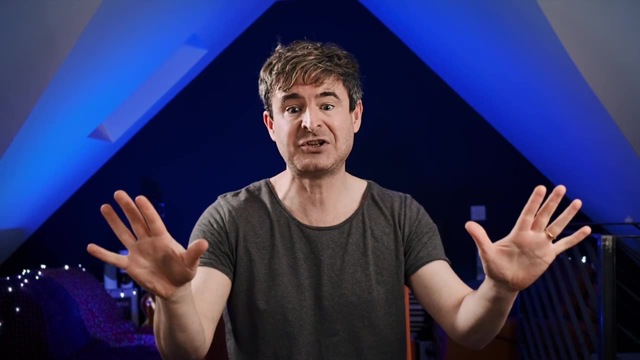 stuff or inferring this stuff from this stuff, but rather to think about the left and the right kind of equally. We accept stuff on the left, we reject the stuff on the right and we're saying if that's a bad situation to be in above the line, then it's a bad situation to be in above the line.